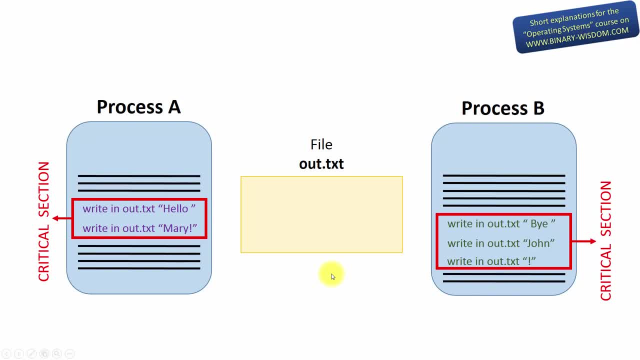 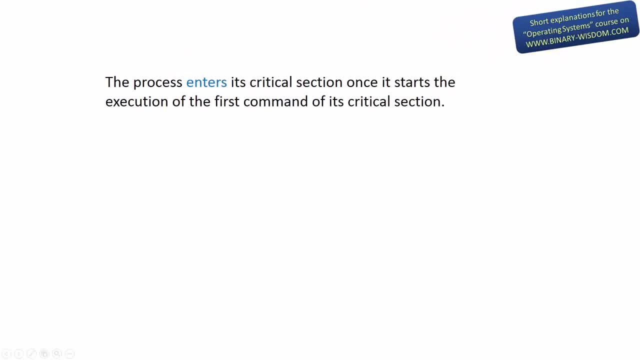 we still consider its critical section running And we still say that the process is in its critical section. To fix this small terminology problem, we can say that the process enters its critical section once it starts the execution of the first command of its critical section. 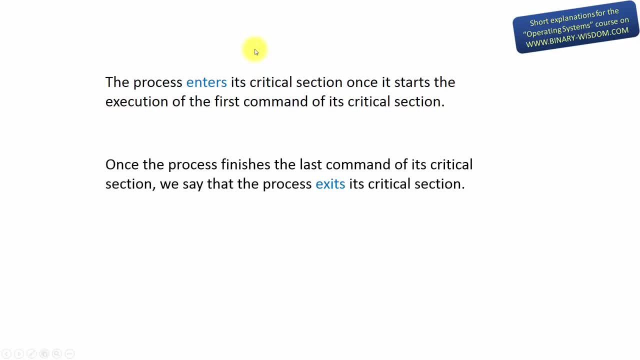 And once the process finishes the last command of its critical section, we say that the process exits its critical section. So if one process has entered its critical section, then no other processes can enter their critical sections until the first process exits its critical section. 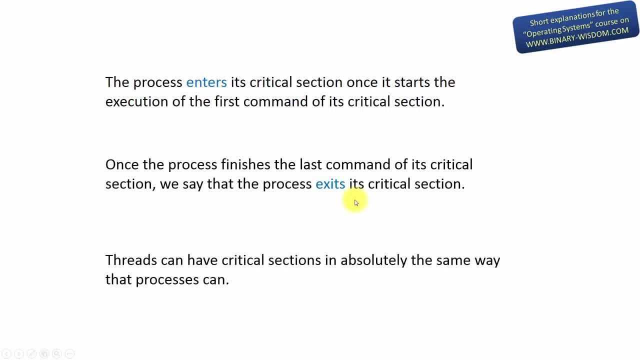 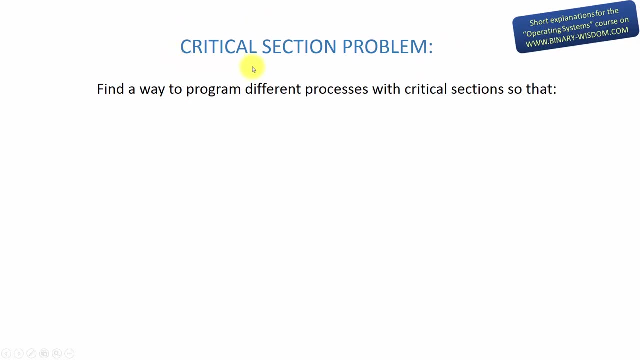 Second, we are discussing critical sections with respect to processes, but threads can have critical sections in absolutely the same way that processes can. Now to the critical section problem. The critical section problem is the problem of finding a way to program different processes with critical sections. 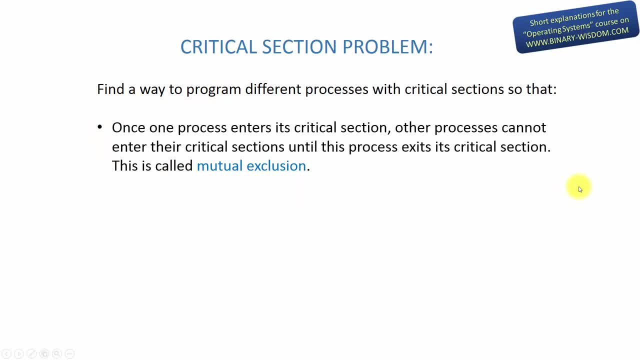 so that once one process enters its critical section, other processes cannot enter their critical sections until this process exits its critical section. This is called mutual exclusion. In other words, don't run multiple critical sections at once When multiple processes want to enter their critical sections. 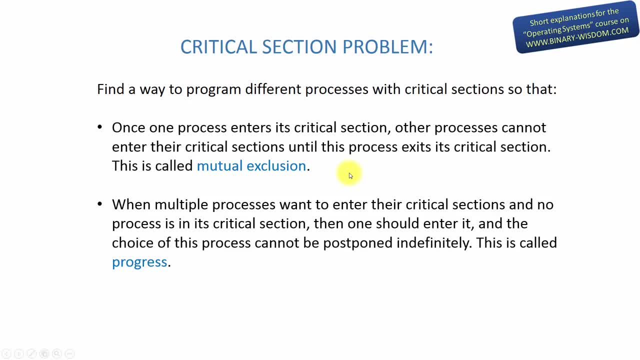 and no process is in its critical section, then one should enter it, and the choice of this process cannot be postponed indefinitely. This is called progress. In other words, keep shared resources busy and avoid deadlocks. No process should wait forever to enter its critical section. 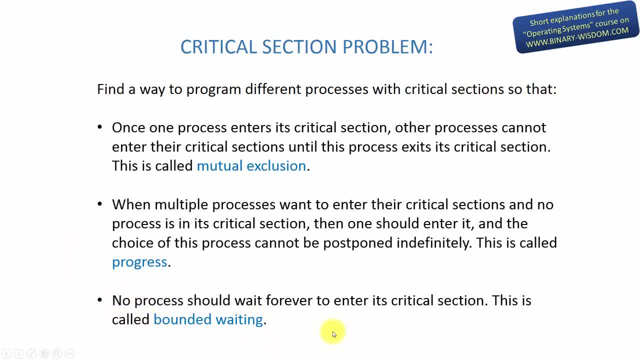 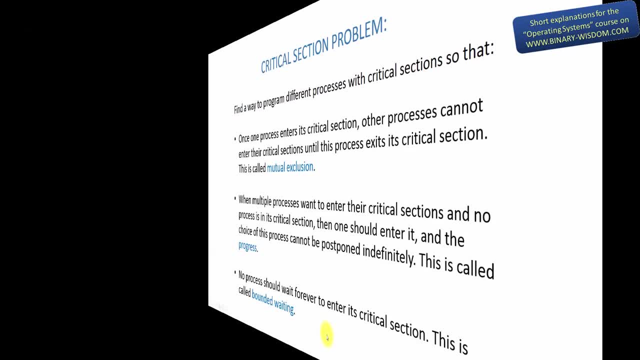 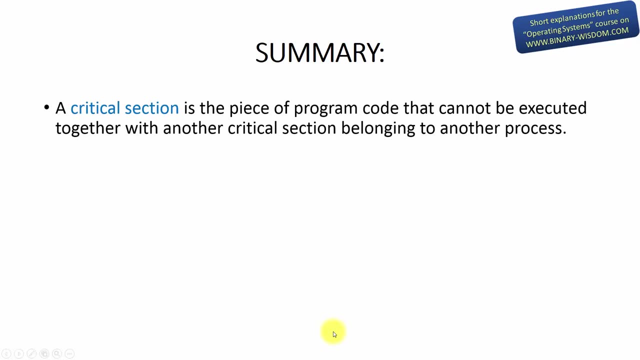 This is called bounded waiting. In the following videos we will discuss tools and techniques to solve the critical section problem. Let's summarize: A critical section is the piece of program code that cannot be executed together with another critical section belonging to another process. 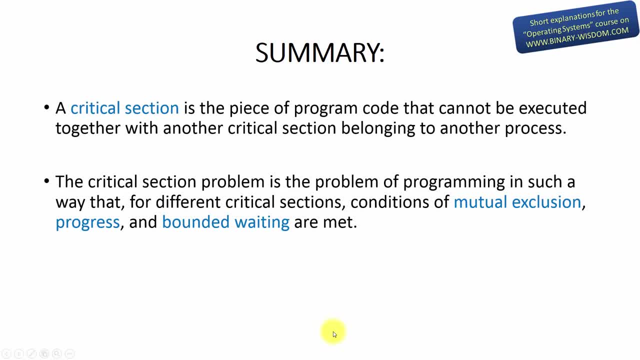 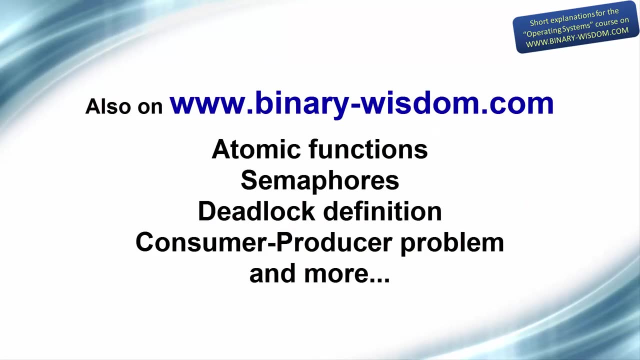 The critical section problem is the problem of programming in such a way that, for different critical sections, conditions of mutual exclusion, progress and bounded waiting are met. That's it. Thank you for being with us. Thank you for watching.